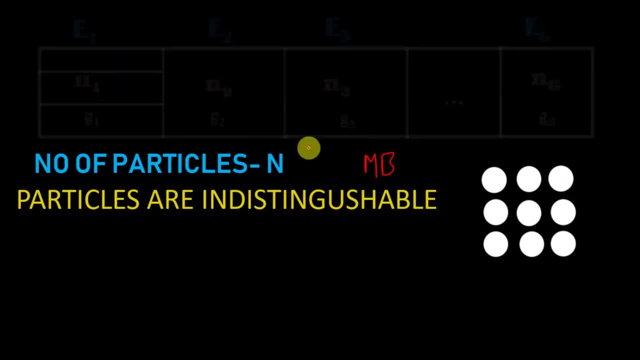 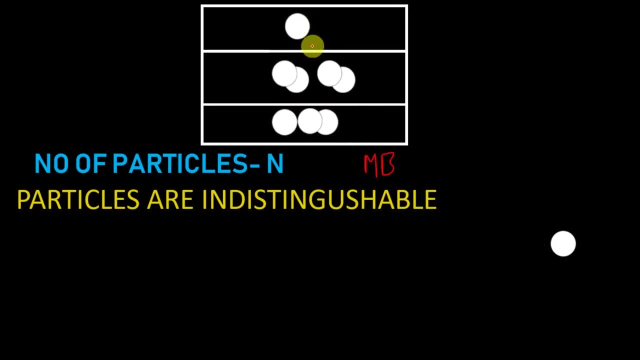 but in here we need to care more about energy levels. So take a look at in here. In here, what we need to care is this: like, how many particles are there in which energy level In here? this particle can go in here and this particle? 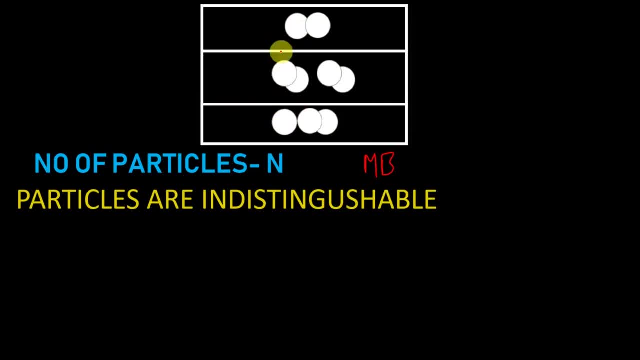 can go in here, but it won't change the microstate, because these particles are indistinguishable. So the only thing that we need to care is that how many particles are there in this energy level, how many are there in this energy level and how many are there in this energy? 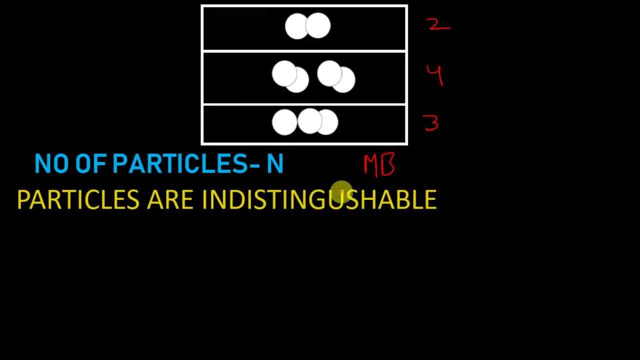 level. This is what we will determine In here. the energy level is not changing in the microstate but in the Maxwell-Boltzmann statistics. changing these two will add another microstate, So in here it makes our task easier than Maxwell-Boltzmann statistics. 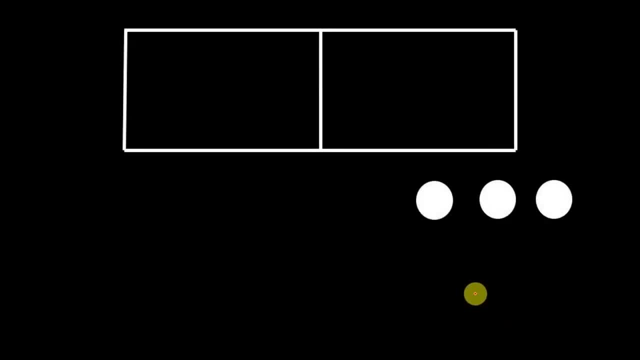 Now what we will do is this: If somehow we are able to find how these Ni particles can arrange themselves in one energy level, then we will get it automatically for all the energy levels. then we will multiply to get our answer. So for simplicity in here I have taken energy. 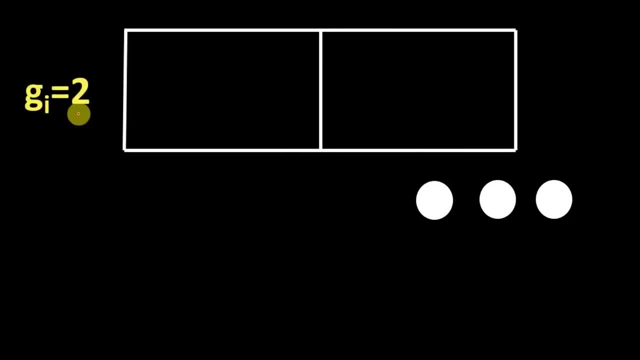 level whose degeneracy is 22.. and now we will try to understand how these three indistinguishable particles can arrange themselves in here. now, for doing that, we will use a really cool mathematical trick. first let me clarify combinations to you first in here, so see if we are like three particles. 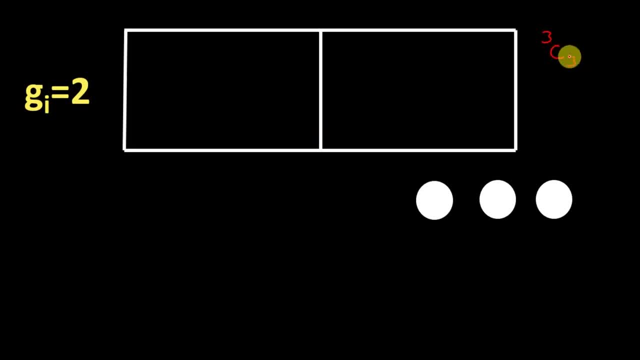 three and we need to choose three of them now. combination is for indistinguishable particles, so which is three factorial divided by three factorial, three minus three, which is zero factorial. so we have one way now. this is the way that we are choosing all three particles now. 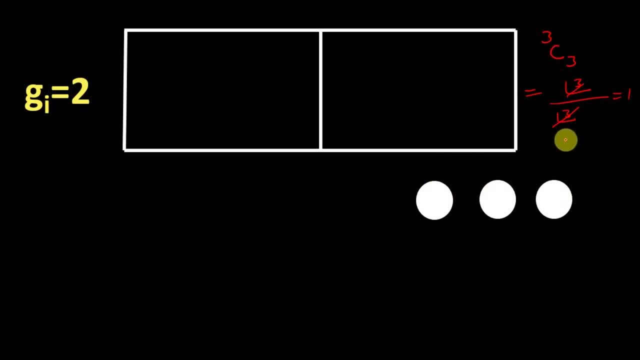 their further arrangement won't count. now, what if we need to choose, like two particles? what will happen then? so we have three particles we need to choose. so two factorial. three minus two is one factorial. so we have three ways. and what are these three ways? we can choose these two particles. 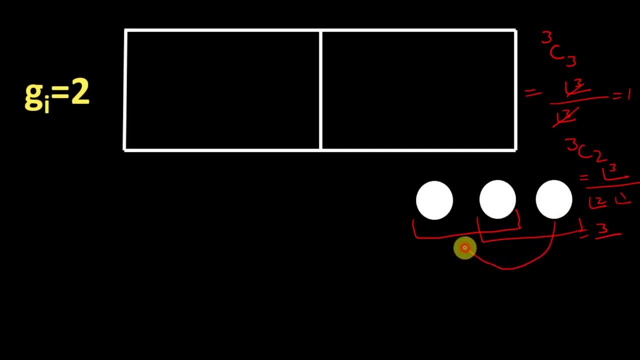 or we can choose these two particles, or we can choose these two particles. so these are these three ways. so remember, in combination, if we have some particles and we need to choose some of them, then, like you are choosing these two or these two, this will count, but choosing these to our 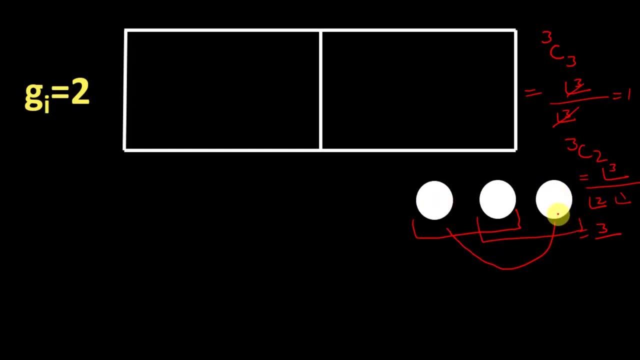 like arranging them: this first, this first, that won't count, okay, so this is really important to understand in here. the second thing that we need to understand in here is that how many lines are there in this particle? those two, you can choose these particles and this will count because the 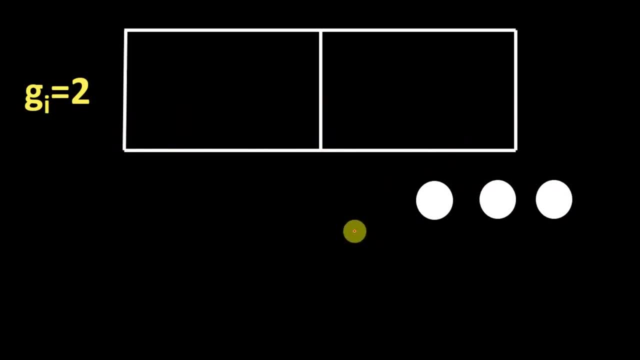 needed in here to create these two degenerate energy levels. So let us understand it. So if we have one line, we have no energy level. If we have two lines, we have one energy level. If we have three lines, we have two energy levels. So to create these two GI, we need GI plus one lines. So 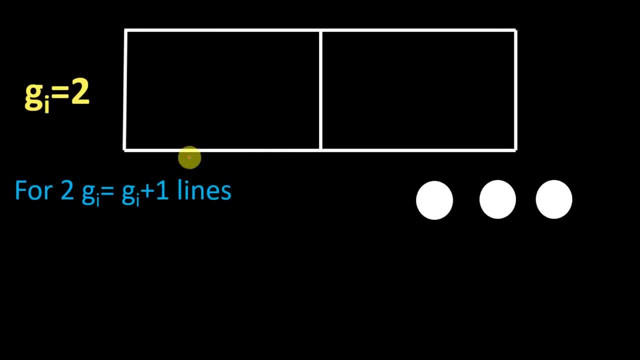 this is general. If we want to create GI levels, we need GI plus one lines. Why I am counting these lines in here? because you have seen that if we choose two particles from three, the waves increase. Okay, so this is really important to see in here. So now let us literally count how these three 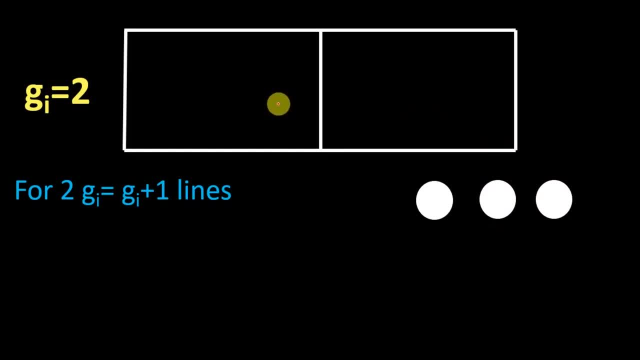 particles can arrange themselves in here. Now you will see a pattern in here. from that we will get our answer. Okay, so these all three can go in here. Okay, now look at this line very carefully. So one particle can go in here. This is another way. Other particle can go in here. This is another. 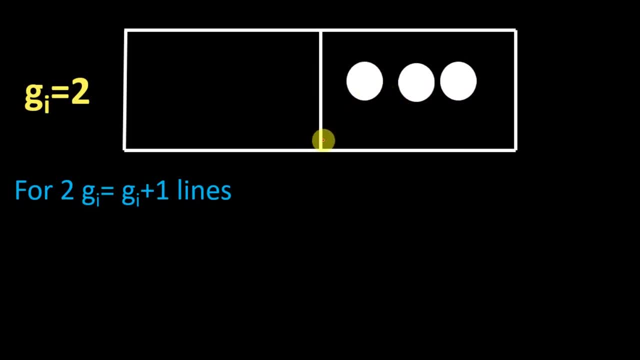 way And then other particle can go in here. This is another way. So we have a total of four ways. So now we need to find this four way, How this four way came in here. Now look at this line carefully. This in here is also acting as an extra. 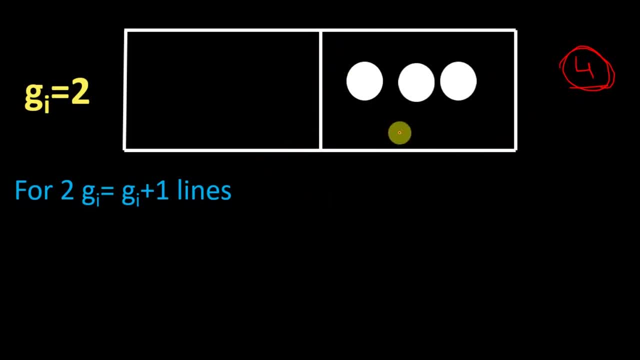 particle, Because let me tell you the answer first, Then we will find how this is. This is like we have four particles- Four- And we need to choose three of them. So we have four factorial Divide by three factorial, And we have in here one factorial, So this is four. So this is how. 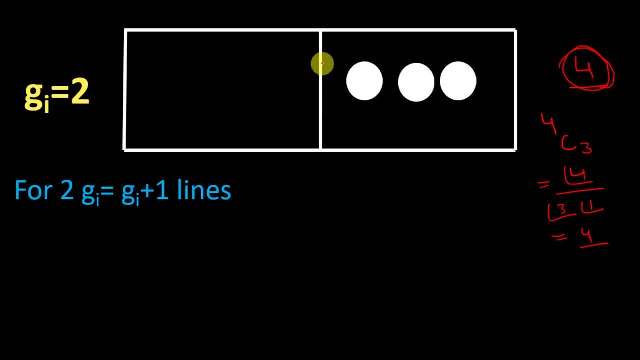 this four came in here. So this line is acting as extra particle And we are choosing three particles from these extra particles. How this is happening, See, at first we have these four particles. Okay, Now we need to choose three particles from them. Which is our Ni? Which is: 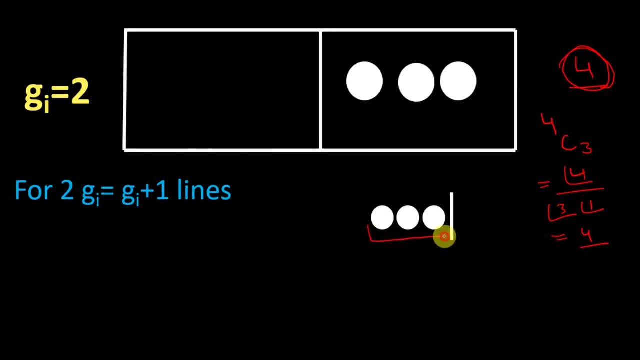 our particles. So the first way we can do is this: We can do this, We can do this, We can do this, We can choose these three. Okay, So we can choose these three. This is our one way. Now we can choose. 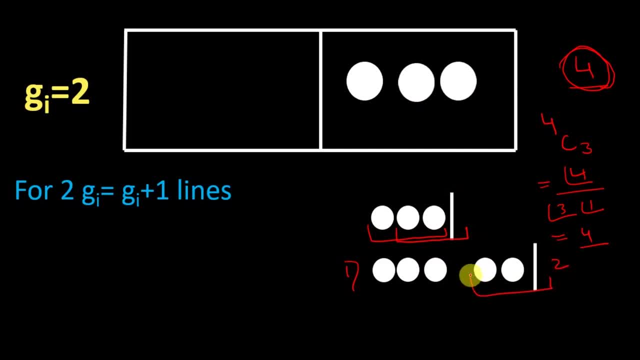 these three. Okay, This is our second way. Now we can choose these three. Okay, This is our third way, And now we can choose this one, This one And this one. This is our fourth way. Also, if we are like a lot of degenerate and level A lot of, And we have a lot of particles also, 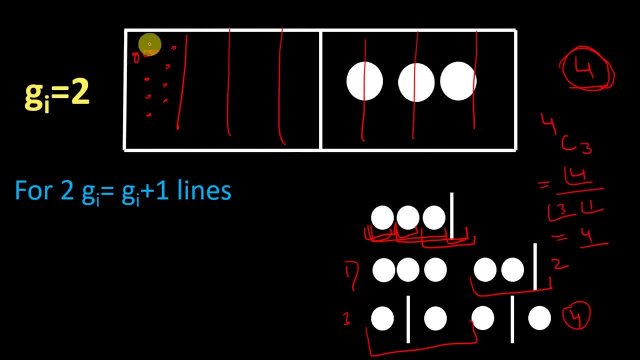 Alright, So the first way will be this one Like. we can select these three And the lines inside lines will also act like particles. So the question will be in how many ways we can select these particles from these all particles Like. the first way will be this one, This one will go. 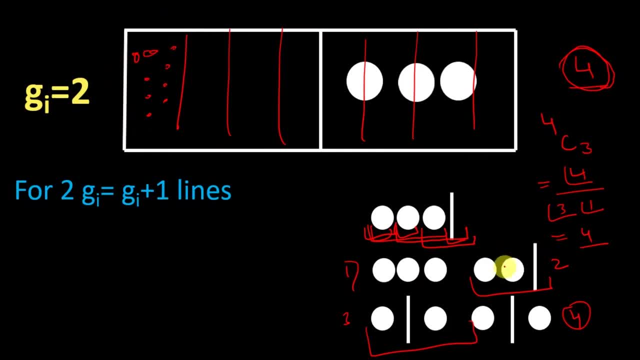 somewhere else. So it will be another way, Like this we have chosen in here. So what we have found in here is general for any Ni And for any other Ni. So this is our third way. So this is an example for any Ga. Now the total number of particles in here, Counting this hypothetical. 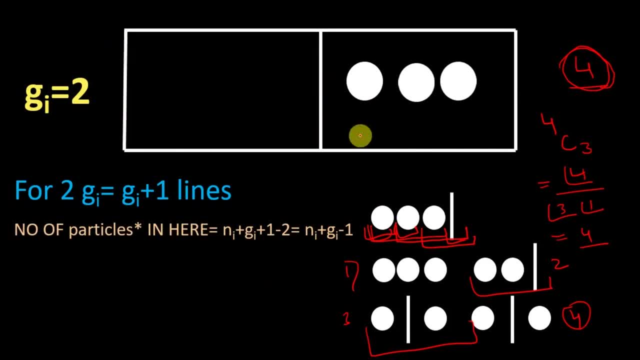 particle. Now I just wanna tell you is that there is no lines thing in nature. It is just a mathematical technique or technique or trick that we are using to find how Ni indistinguishable particles can arrange themselves in Gi energy level. That's it. There is nothing line in. 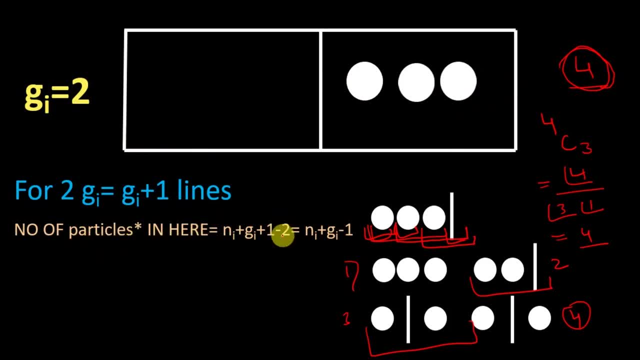 nature. Okay, So the number of particles in here are Ni. These particles plus gi, plus one, that is the number of lines minus two. what is this minus two? minus two is that these and two lines are not counted as particles. these and two lines will be there in every type. 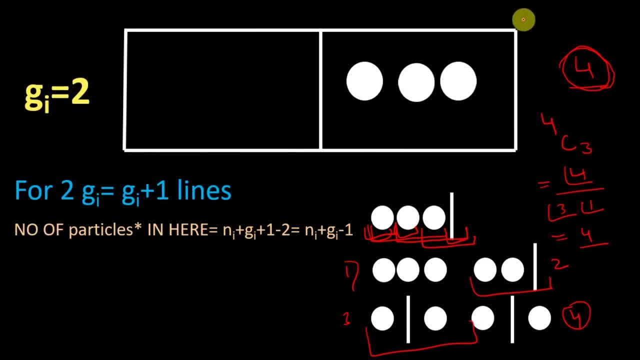 of degenerate and level, like if there are some 10, then these and two lines won't count. so this is that minus two. so the total number of particles in here are ni plus gi minus one. in here it is three plus two minus one, which is equal to four. so from these four particles we need to choose. 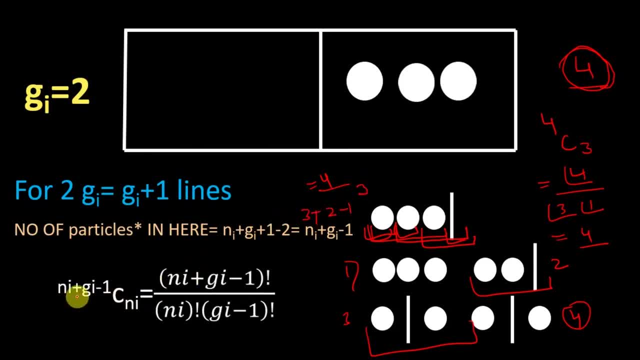 three. so the formula in here is that ni plus gi minus one c and high. we have this number of particles and we are choosing these from this number of particles, which is equal to this factorial, divided by this factorial. this minus this, that is, ni, will cancel. so we have gi minus.